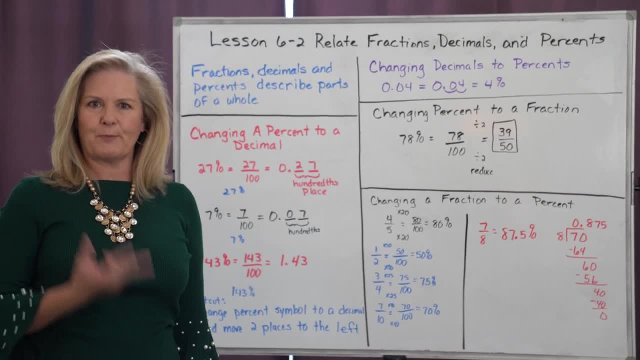 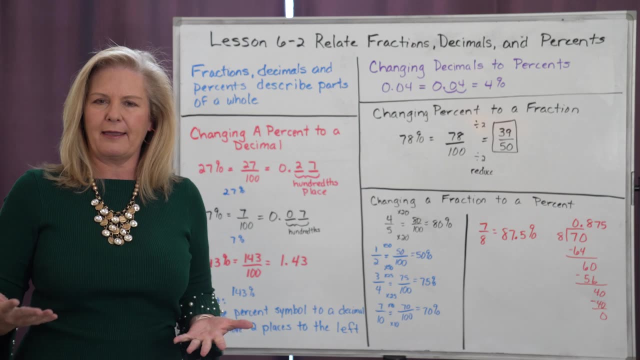 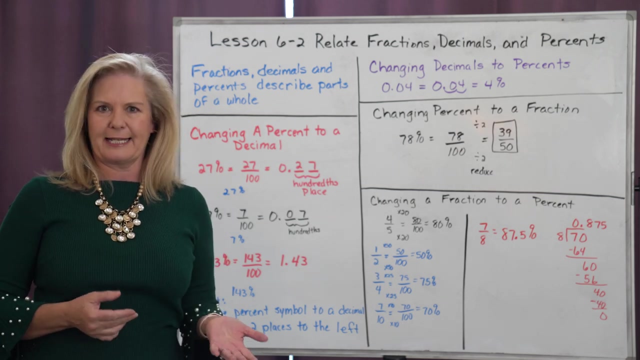 We know fractions, decimals and percents all look at parts compared to a whole, And because they all look at the same thing, I can write any number as a fraction or as a decimal or as a percent, And so what today's lesson is all about is how do we go back and 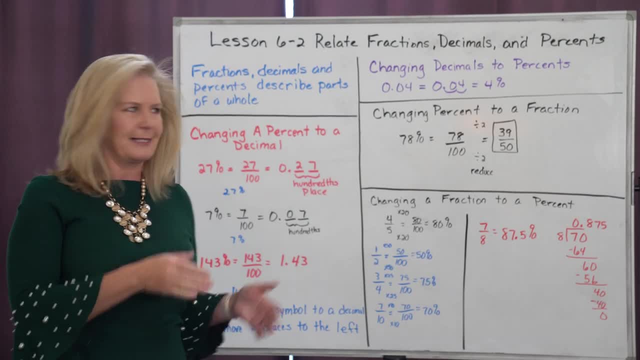 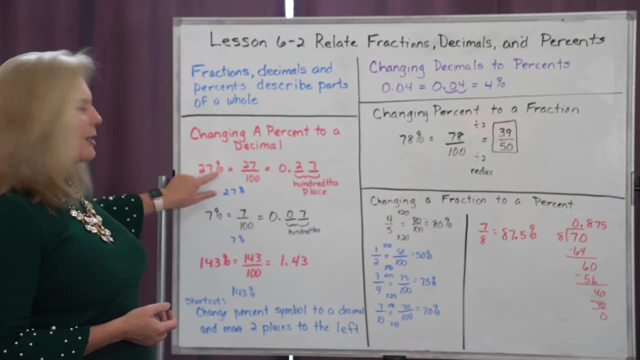 forth between fractions, decimals and percents. Well, the easiest one to do is probably changing a percent to a decimal. We know that a percent simply means out of a hundred. So if I have 27%, it means I have 27 compared to a hundred. Well, that hundredths place right there gives. 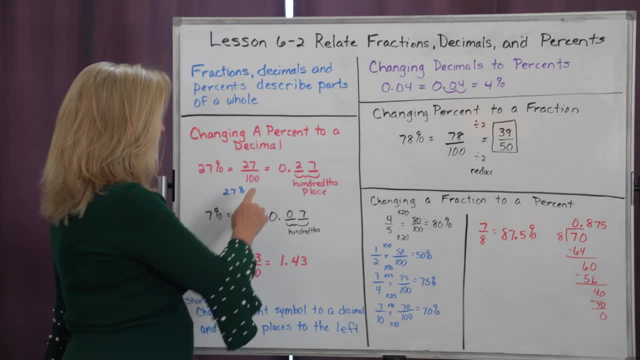 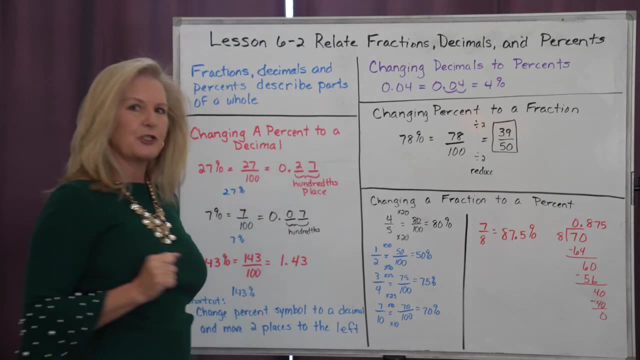 me a place value of a hundredths place, And so if I want to convert this percent to a decimal, all I need to do is go two places to the right of the decimal point to reflect the hundredths place And I take whatever that numerator is and I place it in those slots for the hundredths. 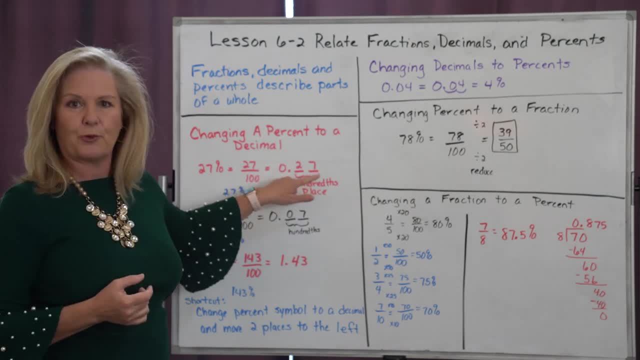 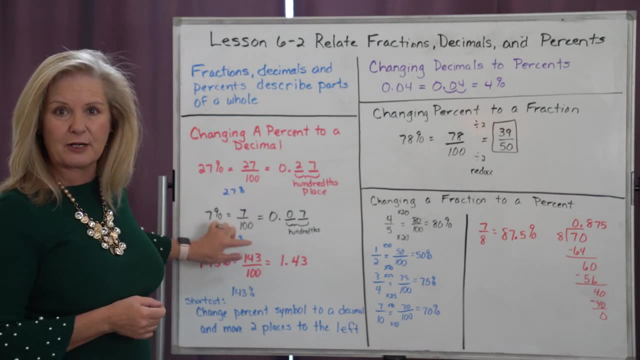 place. So 27% is the same as 27 hundredths. Now we can also do it with single digit numbers. So if I have 7%, that's 7 out of a hundred. I'm still going two places to the right of. 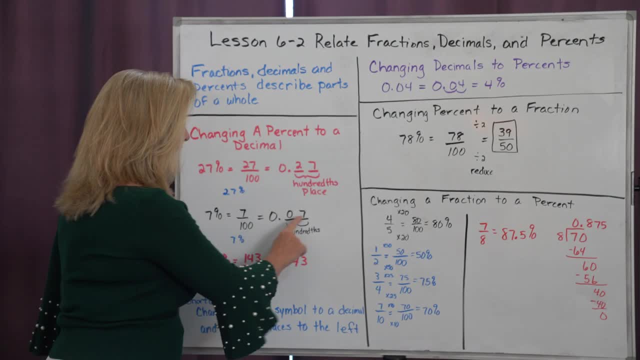 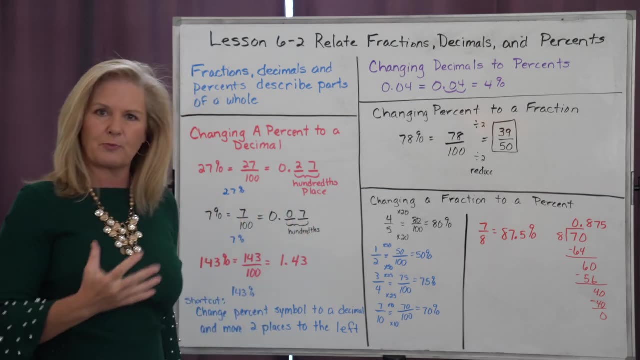 that decimal point for the hundredths place. Now this 7 has to go furthest to the right. So I'm going to put a zero in the tenths place and a seven in the tenths place And I'm going in the hundredths place to reflect the seven hundredths. Now, sometimes we're going to have 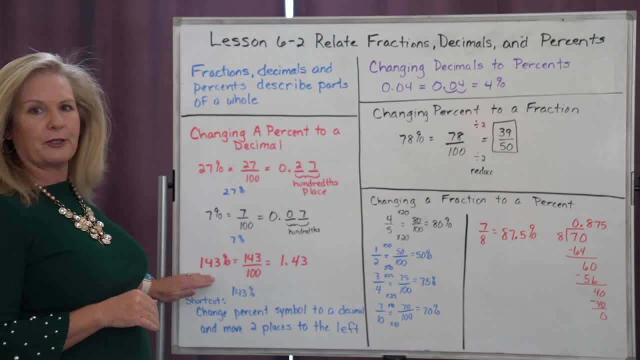 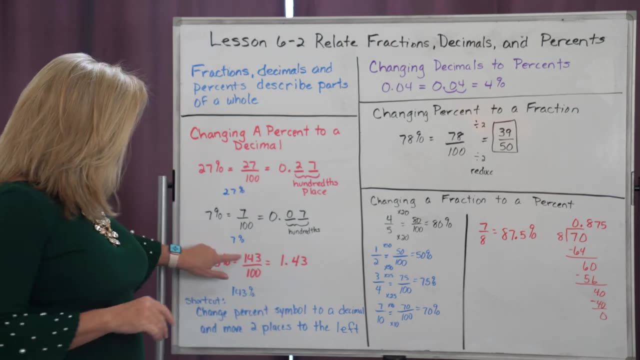 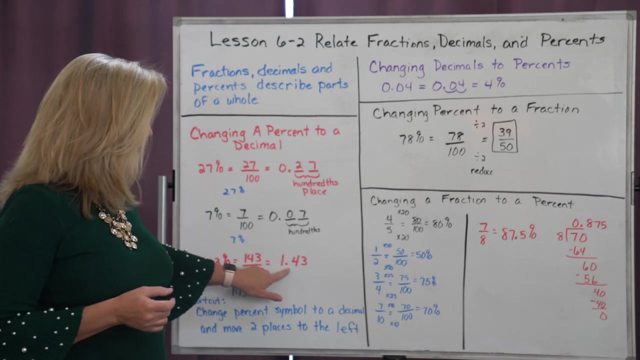 percents that are over a hundred percent, such as 143 percent. Well, again, that's going to be reflected out of a hundred, because a percent means a hundred. Well, if we take 143 percent over a hundred, all I do is I have a mixed number that comes out, I get one and forty-three hundredths. 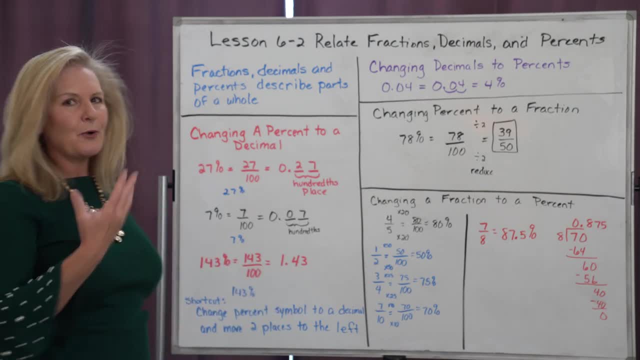 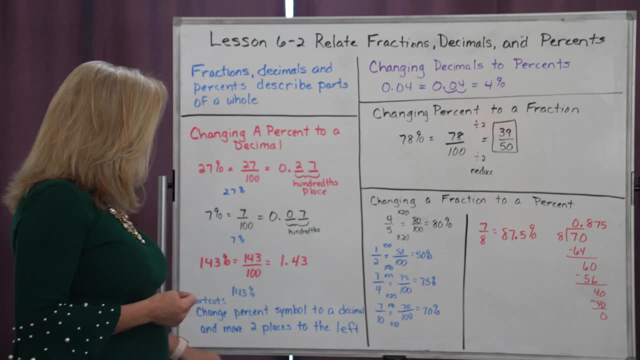 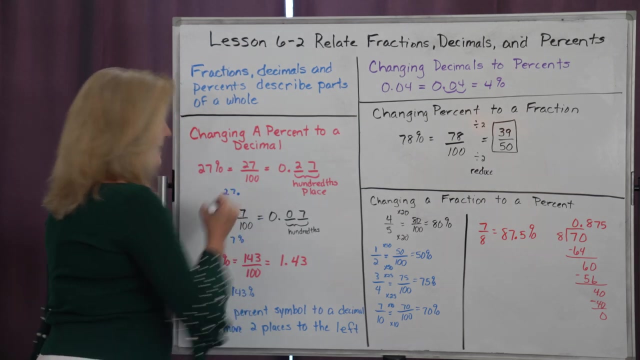 Now there is a shortcut to doing this and most people like to do the shortcut if they understand why the shortcut works And what the shortcut is is. you can take that 27 percent and just erase that percent mark and you're going to replace it with a decimal point And in order to change it, 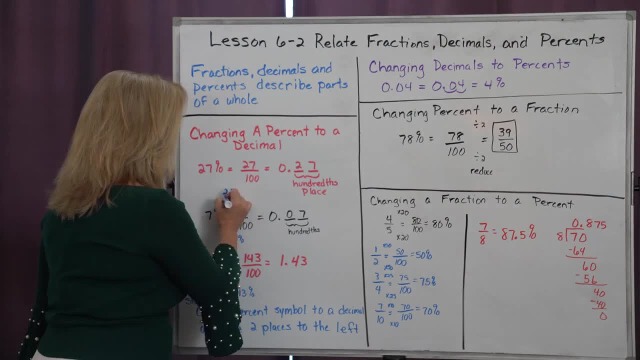 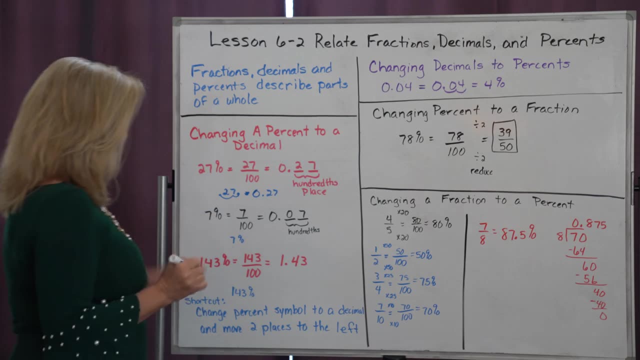 from the percent to the decimal. we just move that decimal point two places to the left and therefore I get zero and twenty-seven hundredths. And if I did that for the seven percent again, I'm going to take that percent out replace it. 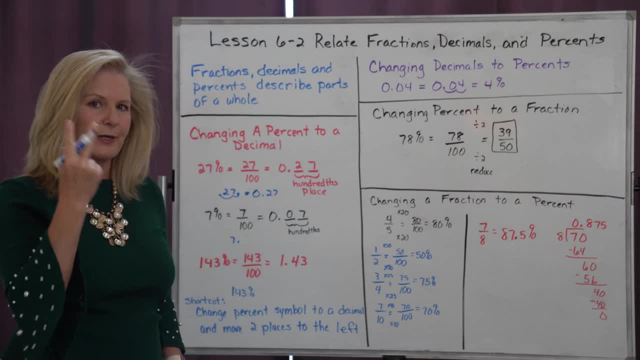 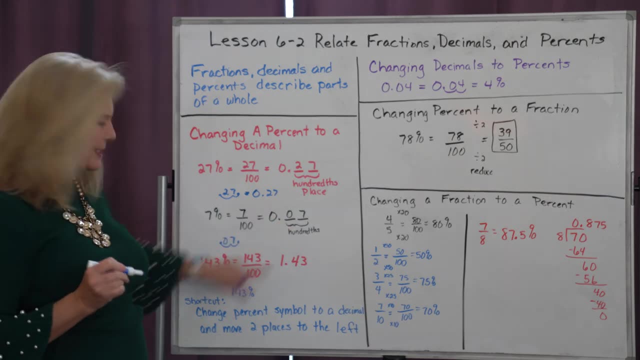 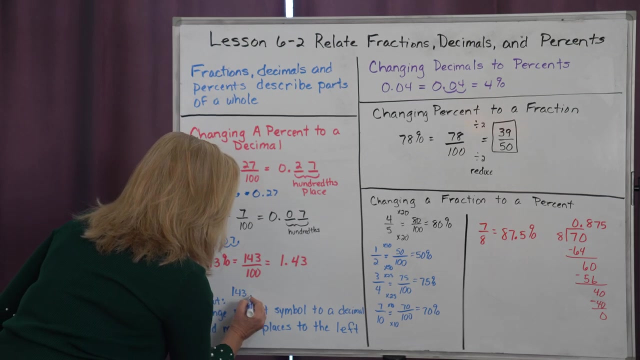 with a decimal but you always have to move it two places to reflect that hundredths. So I move it once, twice, put a zero in and I get my seven hundredths. And again it's really easy to see with 143 percent, because when I replace that decimal I mean that percent and I move my 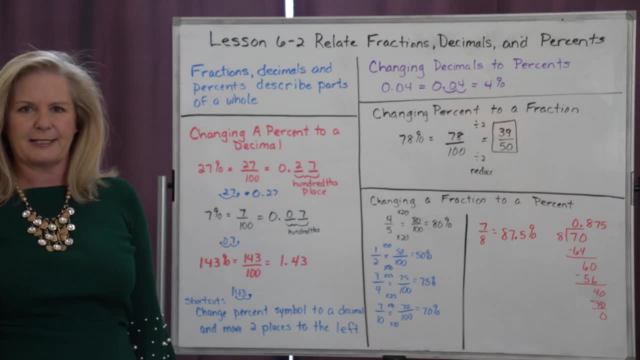 decimal point over there, I get my one and forty-three hundredths. So that's what we're going to do. So that's what we're going to do. So that's what we're going to do. So the easiest is probably taking the percent to the decimal, but we can reverse the direction as well. 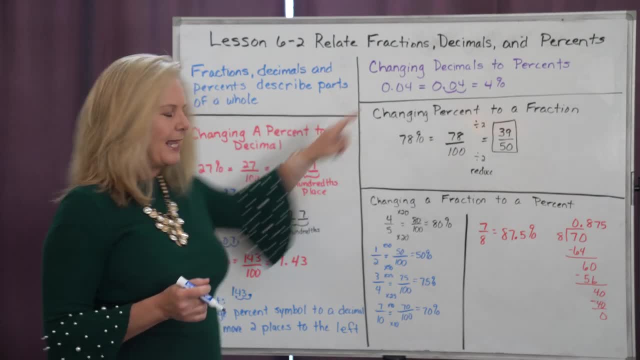 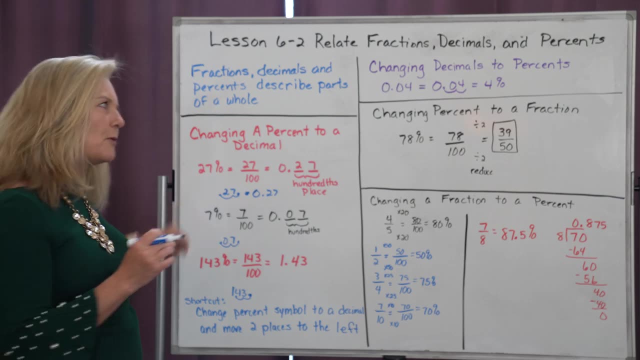 So we can change the decimal back to the percent and it's really based off that shortcut. If we moved it to the left to change the percent to the decimal, all we have to do is reverse it and move it to the right to change it back to the percent. 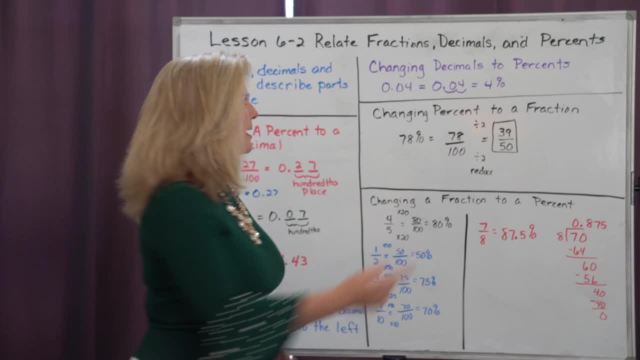 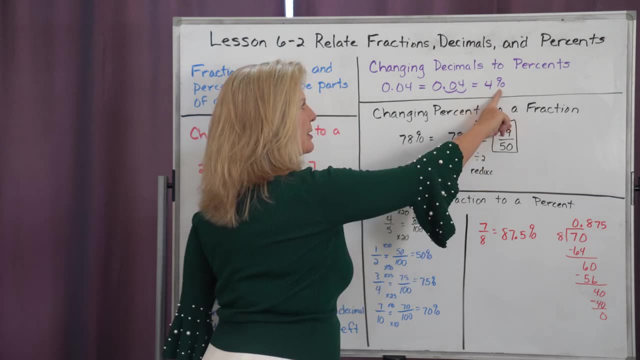 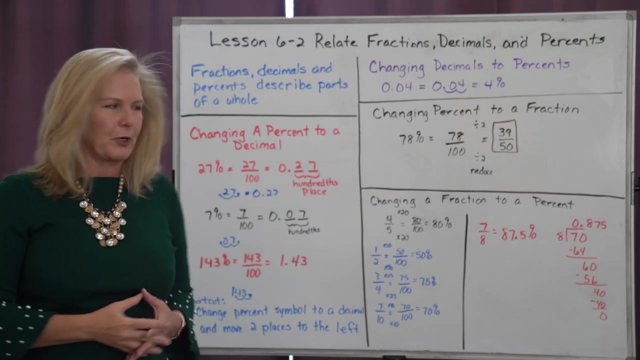 So if I have the decimal four hundredths, I'm going to move that decimal point once twice. then I drop the decimal point, replace it with the percent. therefore I get four percent. So decimals and percents very easy to work with. but we also can change percents and fractions back and forth. 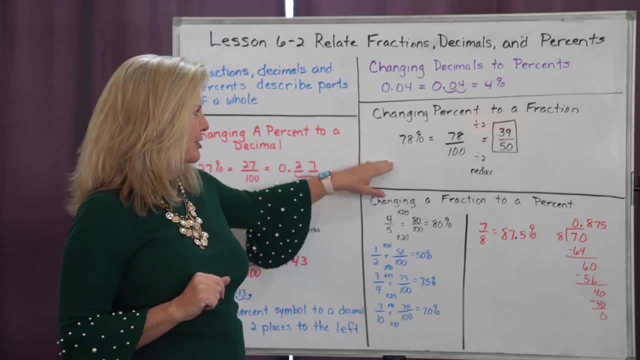 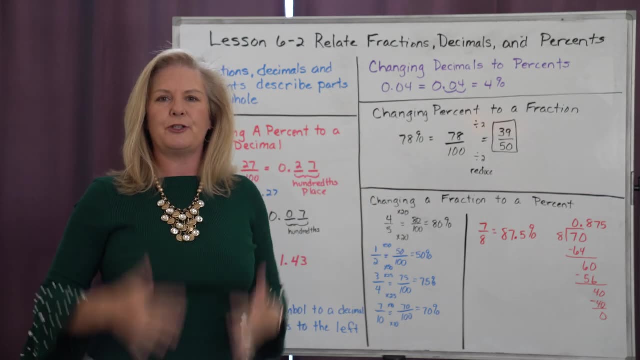 So if I want to change a percent to a fraction, well, we've already done that. Remember that percent means out of a hundred. Now, often we have to reduce that fraction. So if I take my seventy-eight hundredths, 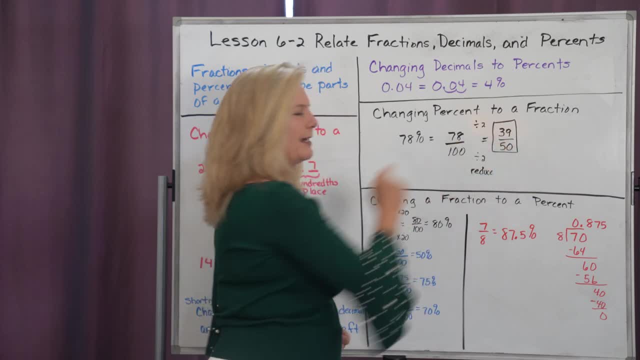 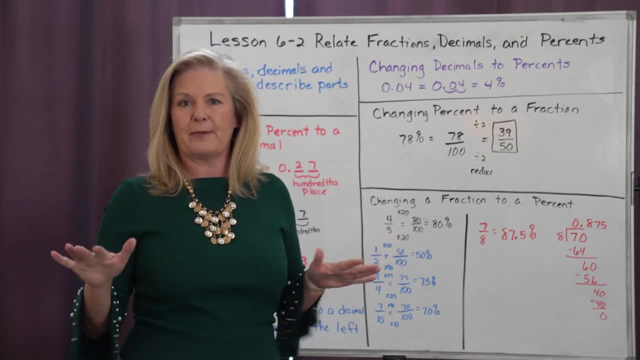 and I divide by two, I get thirty-nine-fiftieths. So seventy-eight percent is the same as thirty-nine-fiftieths. You just need to remember to reduce. Now there are some fractions that are very easy to change to percent. 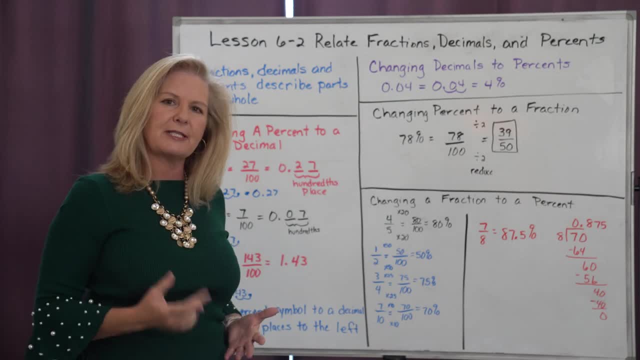 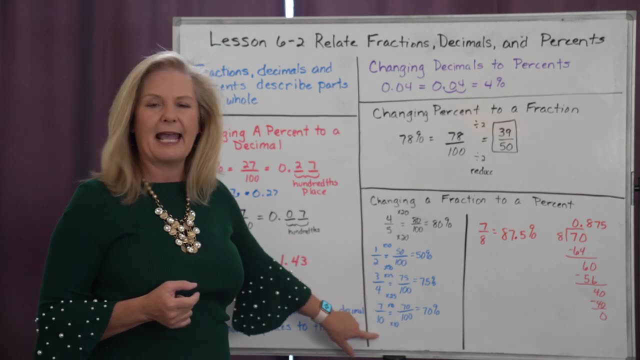 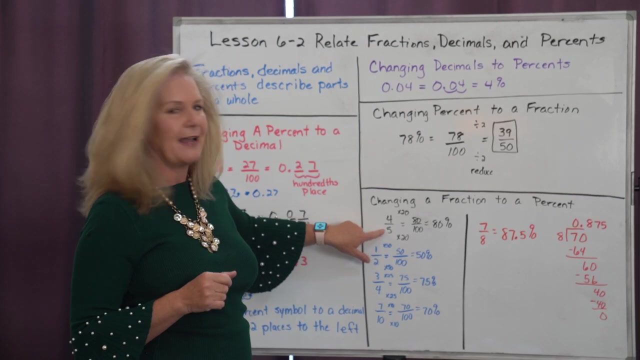 and those are the fractions that have the denominators that are factors of one hundred. So fifths, halves, fourths and tenths are all factors of a hundred And all we have to do is think: if I have a five as a denominator, how do I take that five up to a hundred? 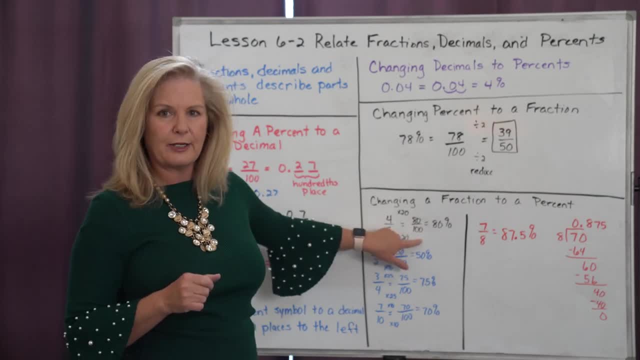 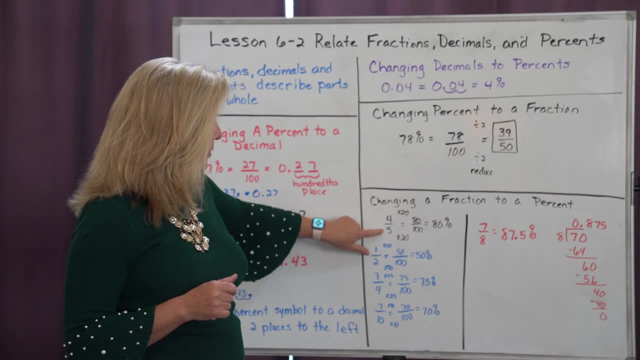 Well, if I multiply five by twenty, it does equal a hundred. But whatever I do on the bottom, I have to do on the top. So four times twenty is eighty. So four-fifths is the same as eighty-hundredths. 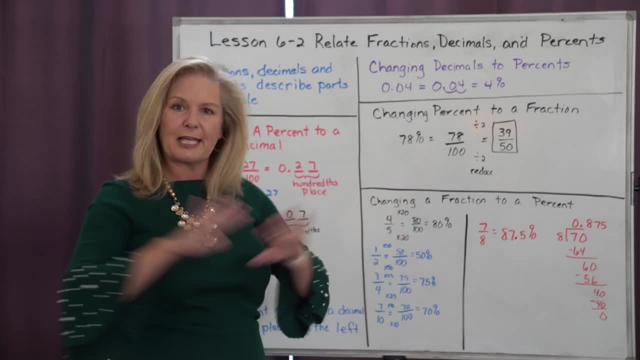 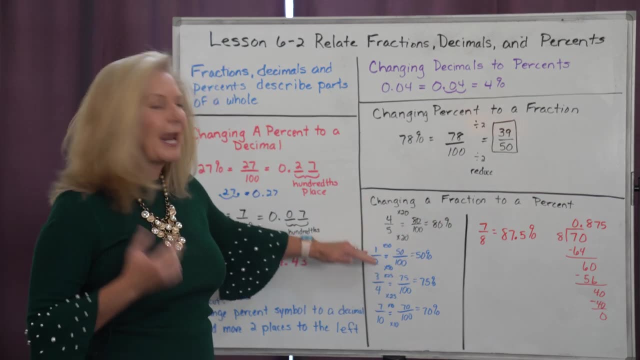 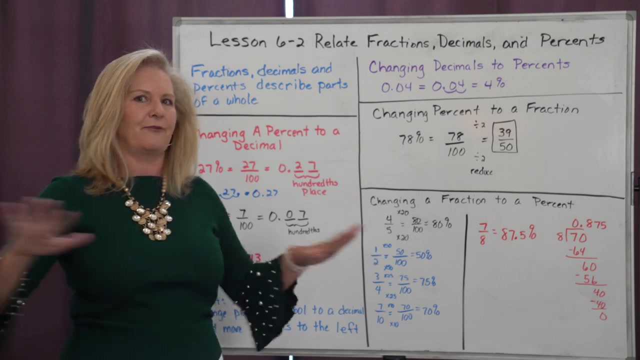 Once I have that denominator of a hundred, I can drop it and I just take the numerator eighty and put my percent, And that will be the same for any fraction with the two, four and ten as well. Now we can have fractions that have different denominators than that. 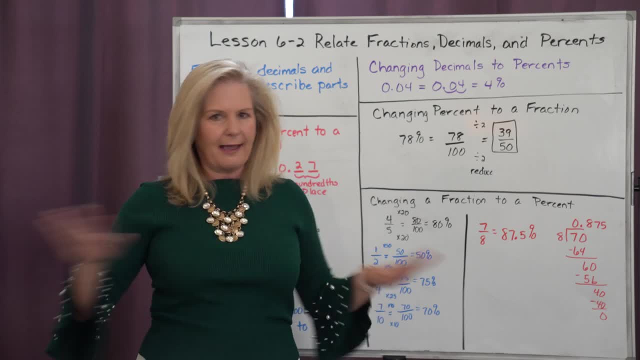 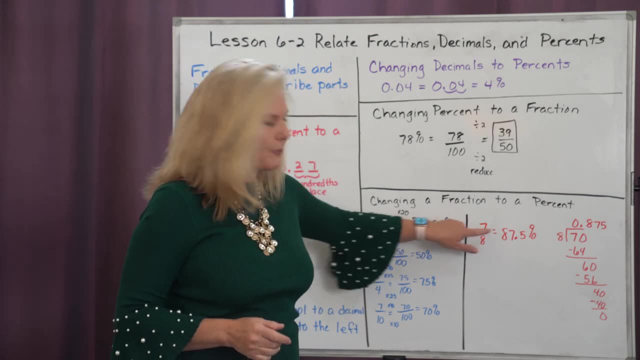 An example would be seven-eighths. Okay, there is nothing. I can multiply eight by. that's going to get me to a hundred. So remember this line right here tells you to do division. So it's really seven divided by eight. 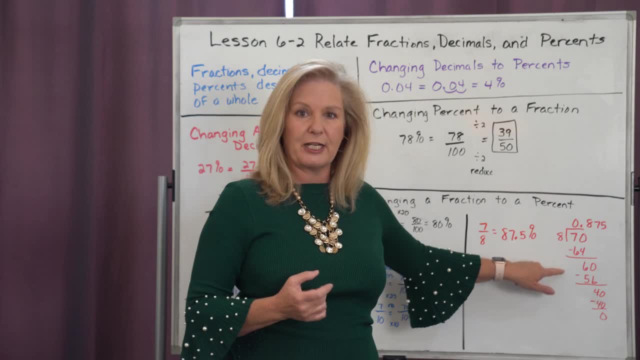 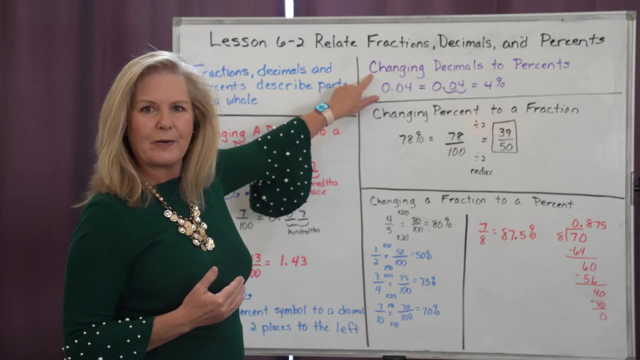 So you can come over here and actually do the division And when you divide it you're going to get a decimal. And remember, once we have a decimal, all we need to do is move that decimal point two places to the right.